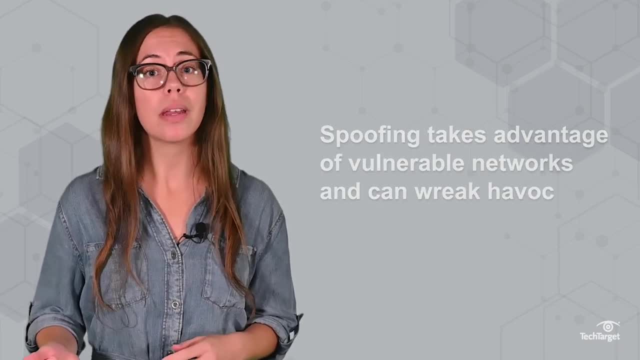 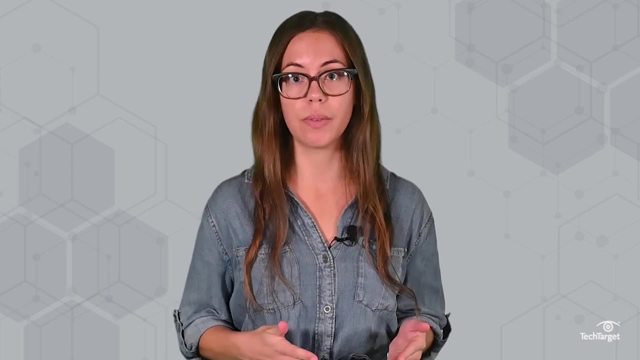 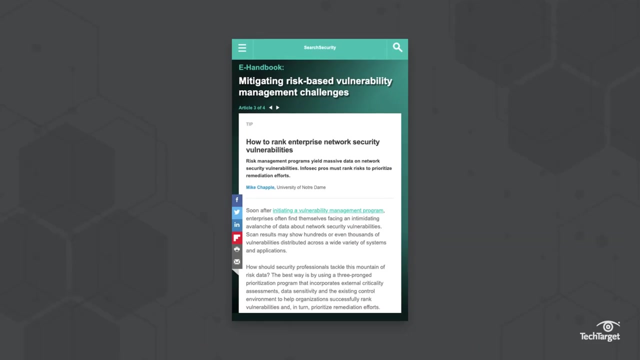 vulnerable networks and can wreak havoc, from collecting company information to gaining access to other network controls. Here we'll cover the most common types of network spoofs To learn about identifying and managing enterprise security vulnerabilities and prevent future attacks. click the link above or in the description below. 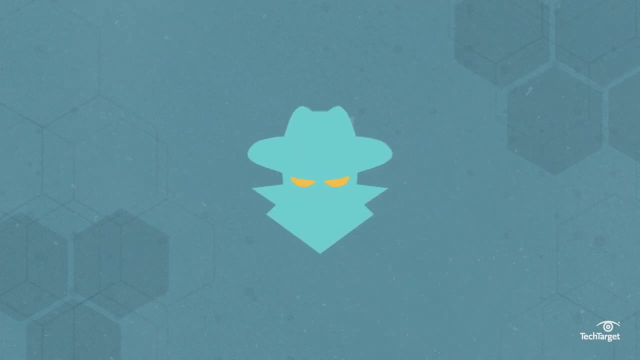 IP spoofing. Internet protocol or IP spoofing is an attack where a threat actor hides a true source of IP packets to make it difficult to know where they came from. This allows attackers to discern, find or track the source of the IP-packet. If a threat actor accidentally hides a source of IP-packets but can't find lost IP. they cannot identify the source. This allows attackers to detect the source of the IP-packet and the most important link in general. This allows attackers to identify and manage the source of IP-packets without the need for the process. the IP address on data packets to impersonate a computer, a sender's identity or both. Spoofed IP addresses enable attackers to keep authorities from finding out who they are, prevent compromised devices from sending attack alerts and bypass security scripts and services. 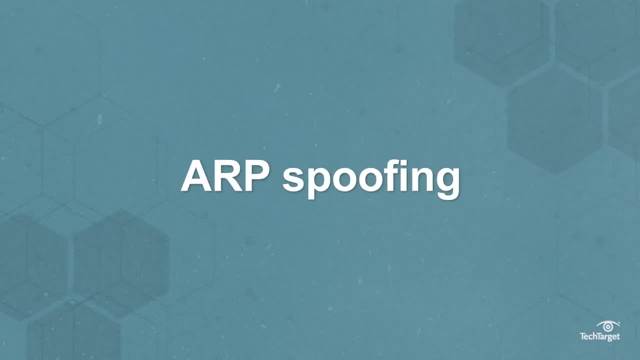 that would have otherwise blocked malicious traffic. ARP Spoofing- An address resolution protocol spoofing attack occurs when an attacker sends false ARP messages over a LAN, linking the attacker's MAC address with the IP address of a legitimate computer or server on the network. 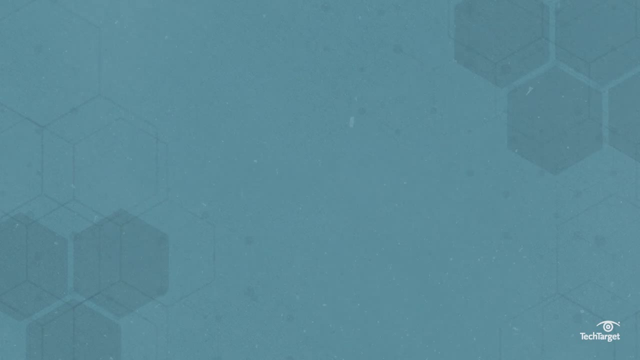 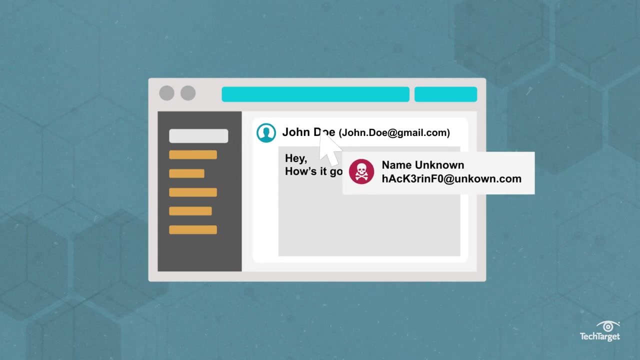 DNS Spoofing- Domain name system spoofing attacks happen when attackers inject fake DNS entries into the DNS servers so that when legitimate users access the server, they are sent to the attacker's injected location, Not their intended destination. Email Spoofing: Here attackers alter email header fields to misrepresent who the real sender is. 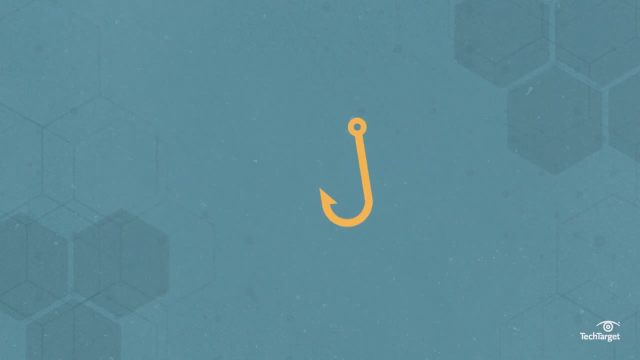 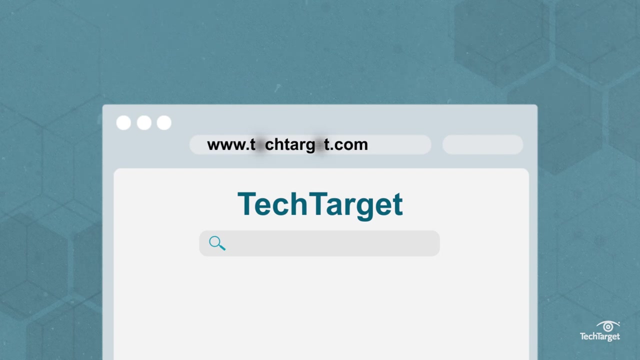 Email spoofs are often used as part of a phishing attack, where victims trust the source of the email and then are tricked into clicking a malicious link. URL Spoofing: With URL spoofing, threat actors use a URL almost identical to a real one, with just a few changed characters. 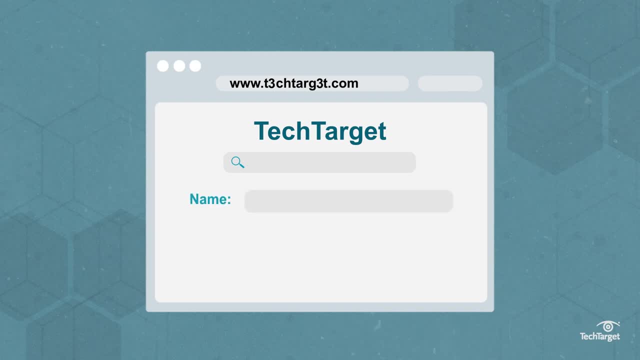 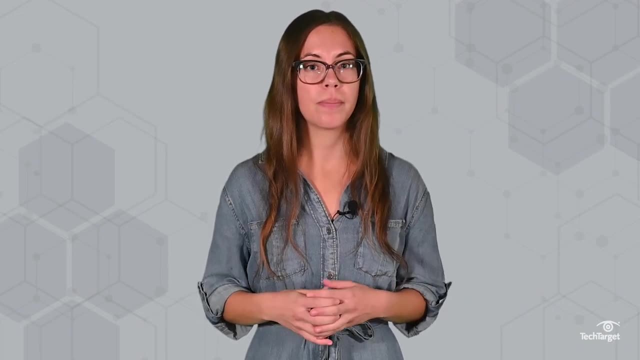 The intent of the spoofing is to make the sender feel like he or she is the real sender. The intention is to get victims to go to a web page that mimics a legitimate one and provide sensitive information. Have you ever fallen victim to a network spoofing attack? 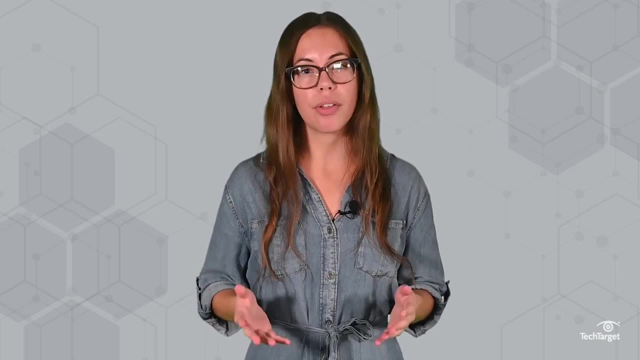 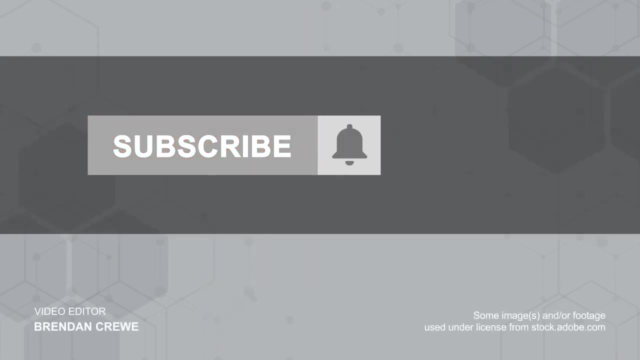 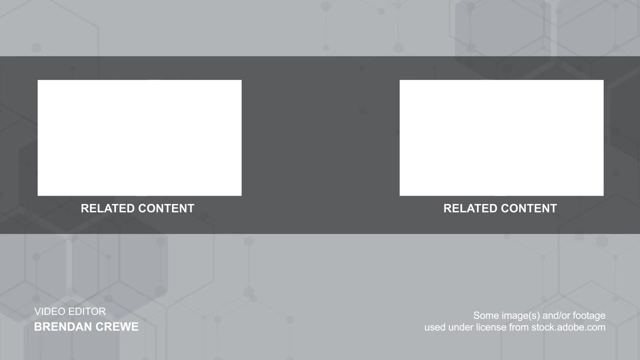 How is your enterprise prepared against spoofing attacks? Share your thoughts in the comments and be sure to like and subscribe. Thanks for watching. 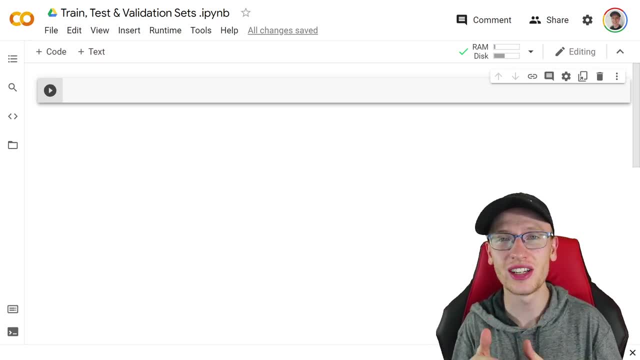 Hey everybody, how's it going? I hope you're doing well today. So this video is on train test and validation sets, a very important concept in machine learning, And if you do not know it already, I highly recommend you stick around and watch this because, no matter what,